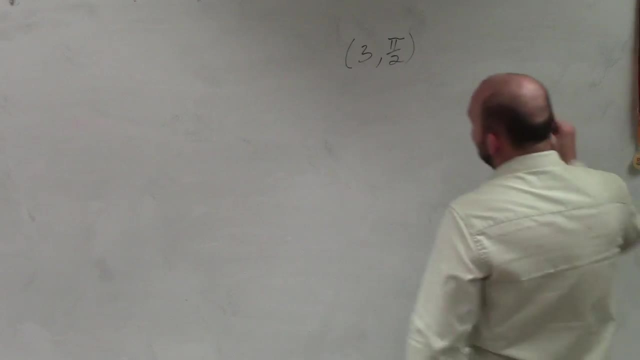 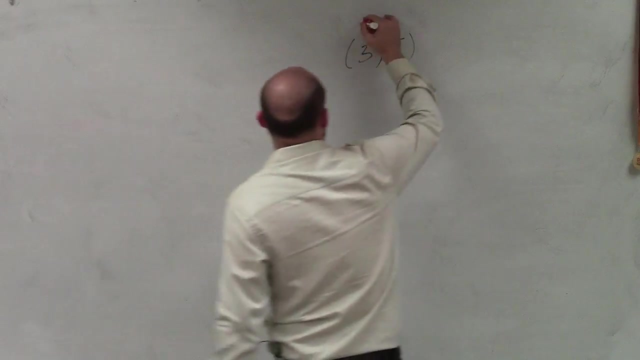 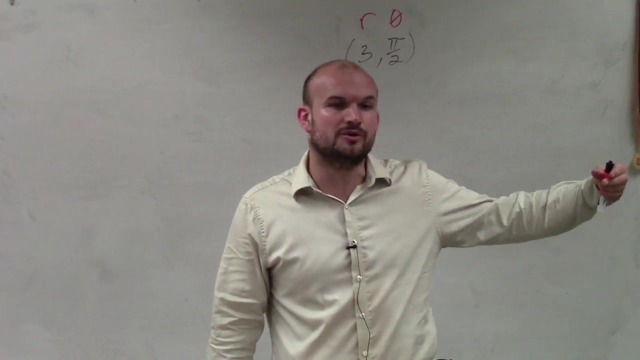 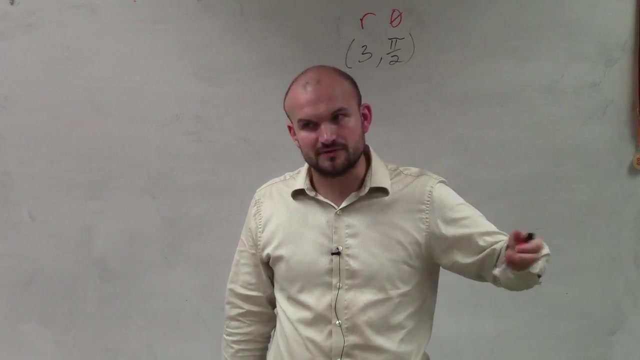 Okay, so if here's our polar coordinate, right? We understand, Zoe, that when we're looking at polar coordinates we have r represents the radius and here represents theta. Now one thing that might be helpful: when you're trying to convert this to your rectangular coordinates, your x and y, it might be helpful sometimes just to look at what does the graph look like for this. 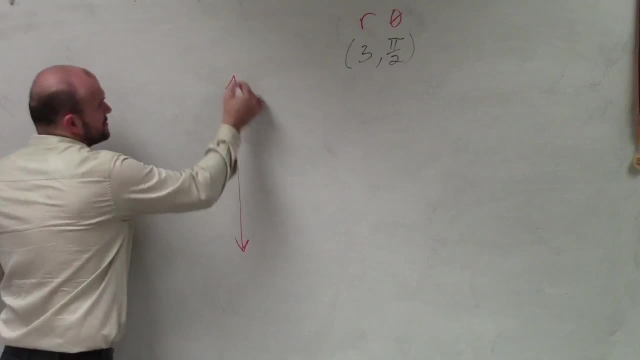 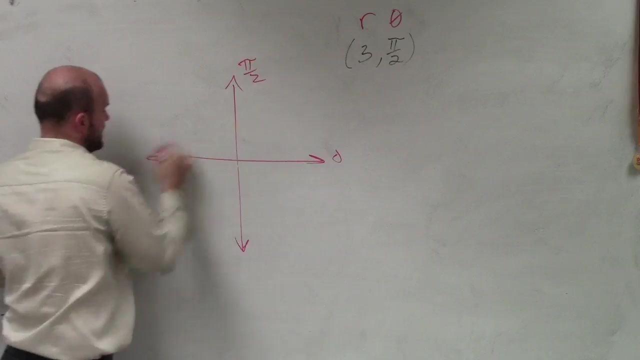 So you don't have to do this. This is a little extra work, but as we're trying to learn through this, I want to show it to you. So again, remember, when we're dealing with our polar coordinate system, we have zero, pi halves, pi three, pi over two, and then we have our lovely unit circle that we start with right. 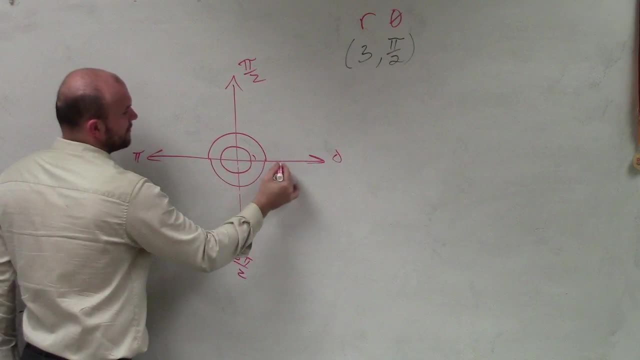 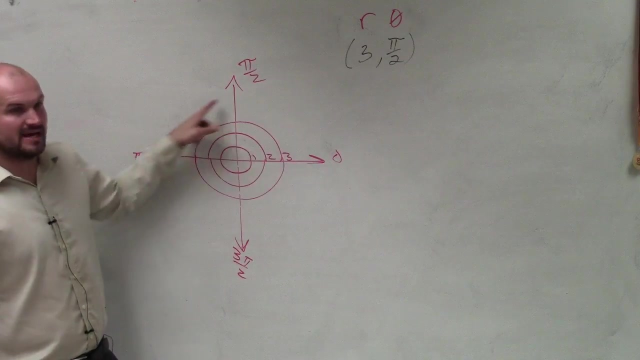 But this one has a radius of three, so it's going to be three rings that we're going to go out, Okay. So remember, the radius tells us three, so that means we're going to, We're going to be on this outer ring and then the angle is pi halves, so it's going to be up here. 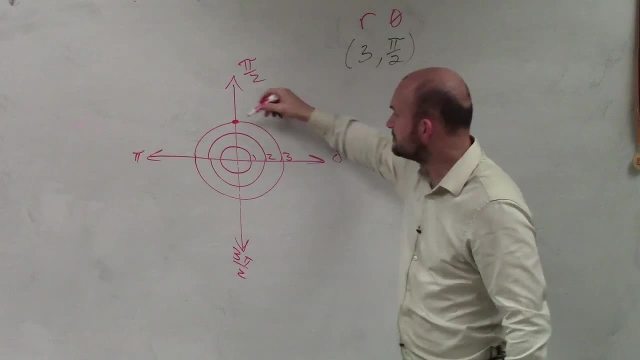 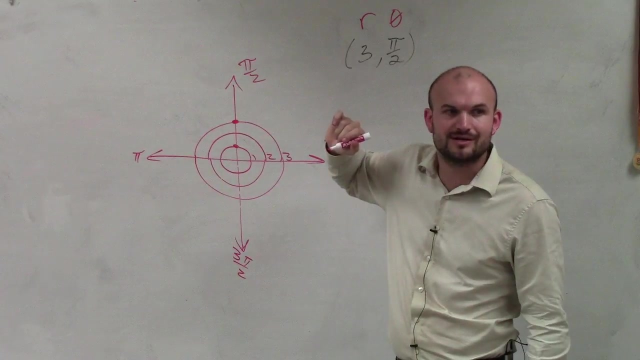 Now, if you guys go back and think about this, all right, here's my angle. at pi halves, What was the x and the y coordinate on the unit circle at pi halves? Does anybody want to raise their hand to remember that? At pi halves, what was that x and y coordinate? 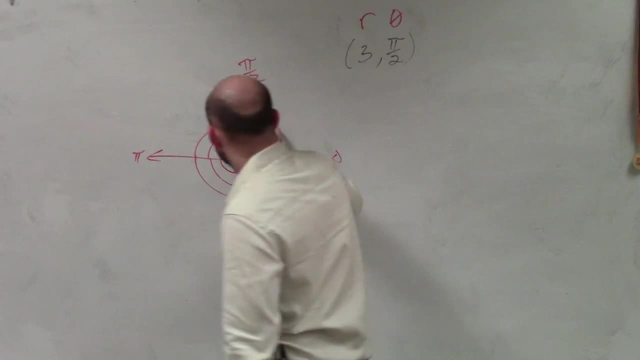 Yes, Kristen, Zero comma one. Very good, All right now I don't want to get through this. but, guys, if I don't get through this, I'm going to be on this outer ring and then the angle is pi halves. 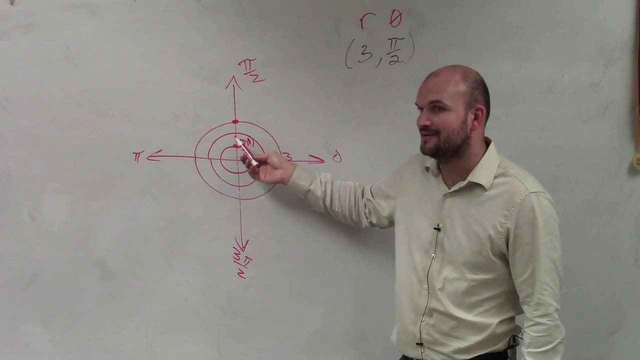 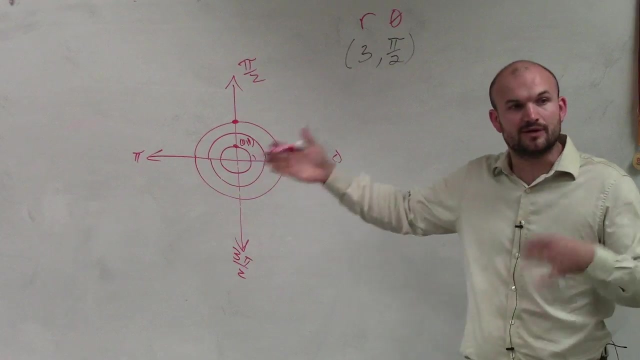 So it's going to be up here. So if I just go up the rings, zero comma one, this would be zero comma two and this would be zero comma three. right, However, let's go back also with the math, just in case, if it's not as obviously known as here. 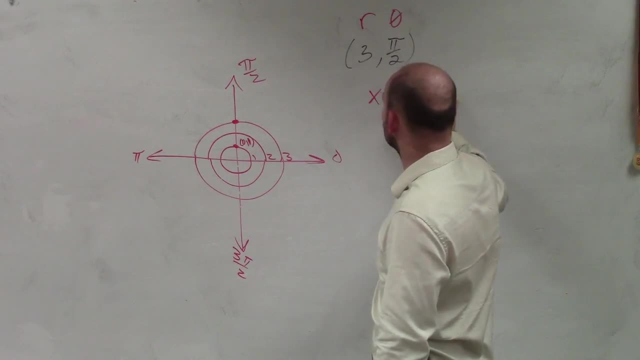 we can still use the formulas. The formulas that we use is: x equals your radius times the cosine of theta, and y equals r times the sine of theta. So let's just go and plug it in real quick, just so we can see why that works with this. 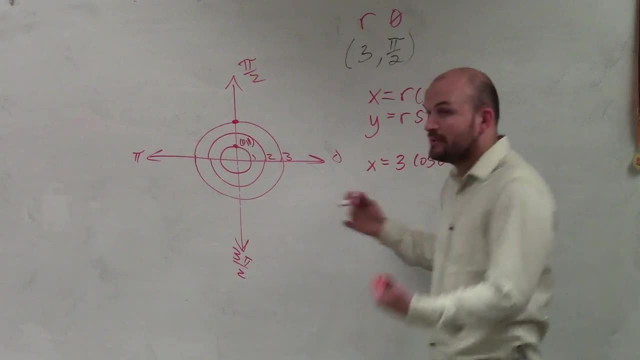 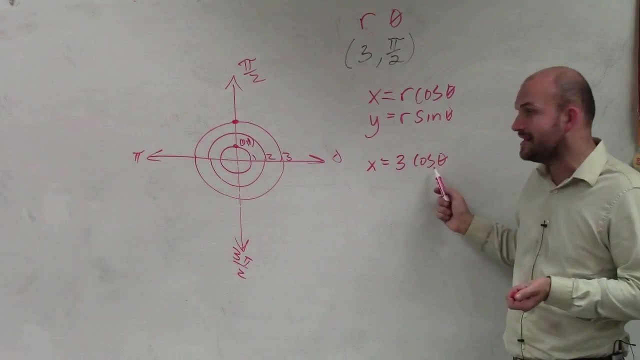 x equals radius, which is three times the cosine of theta. Remember, the cosine of theta is based off of what that unit circle, when you have the unit circle, when you have your radius, is one. So cosine of theta- I'm sorry, cosine of pi halves- is one right.